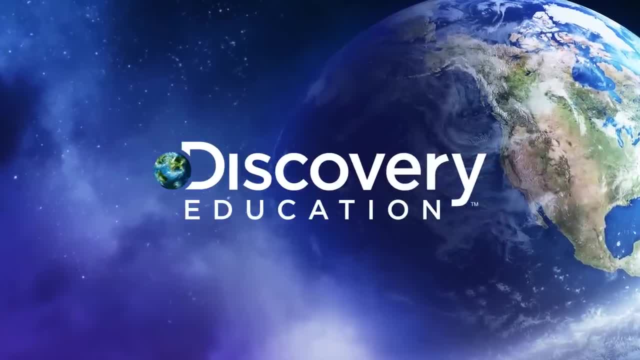 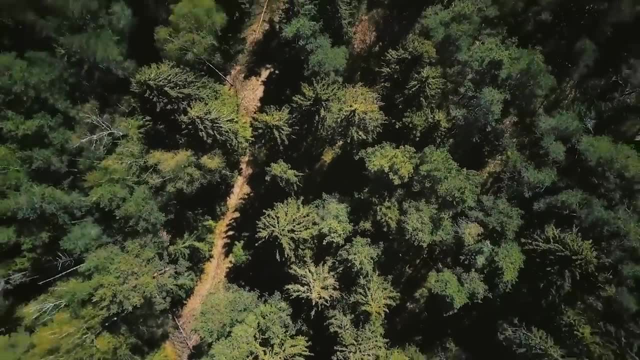 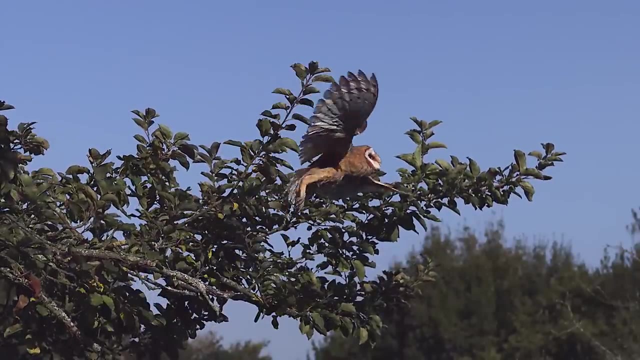 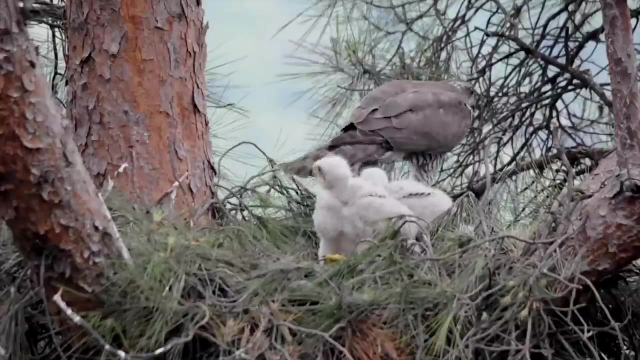 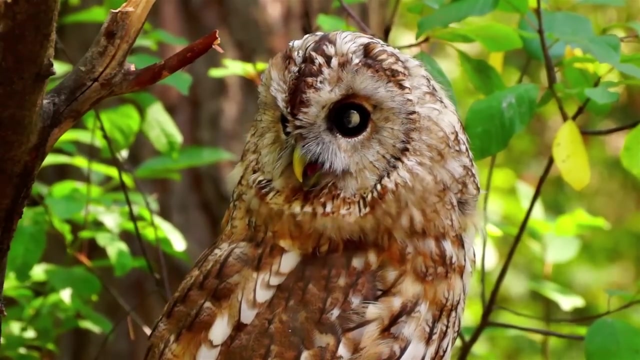 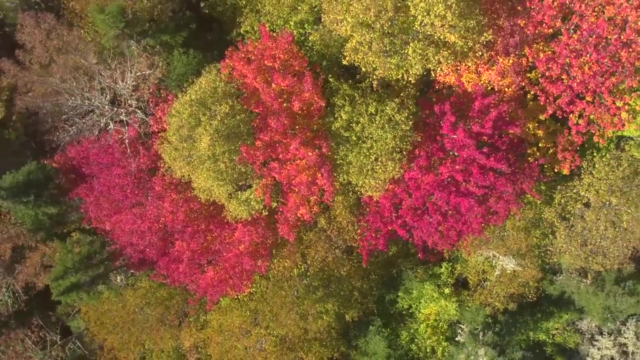 If you were a bird looking to build a nest, where would you make your home? Nestled in the branches of a tree, Hidden from predators? Woodland habitats provide shelter and food for a great range of animals and plants, A habitat that changes as the seasons pass. 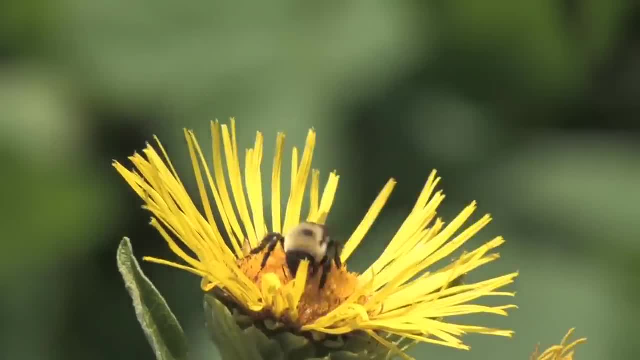 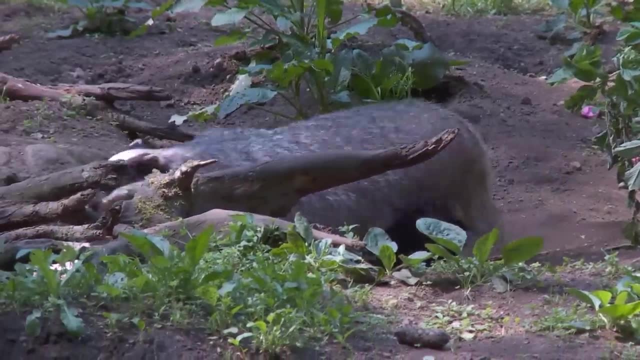 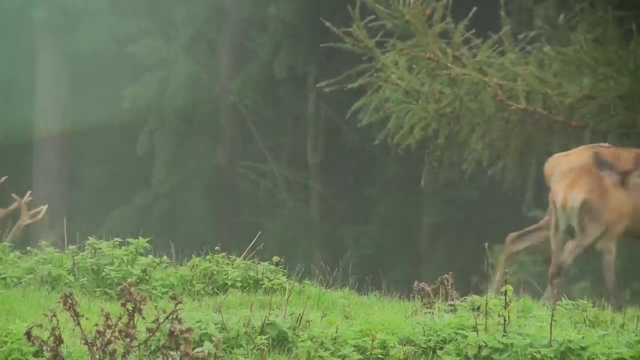 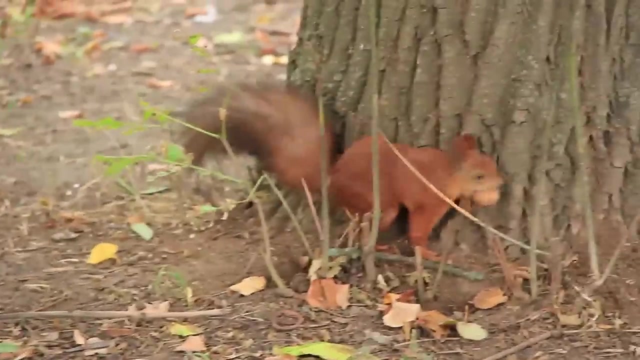 Winter, Spring, In the early summer, a new generation of young are thriving with the abundance of food. Deer take their first steps within 20 minutes of being born. Autumn brings a blaze of colour to the trees And with it a natural harvest of acorns, sweet chestnuts and berries. 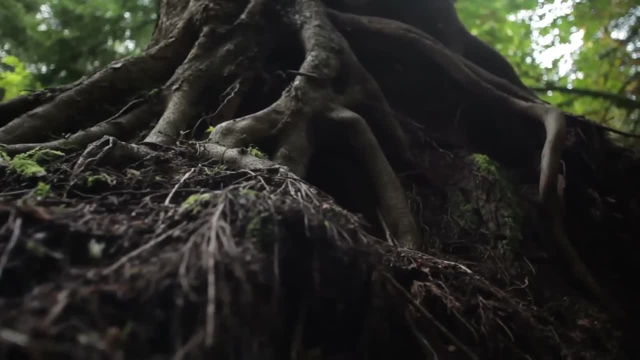 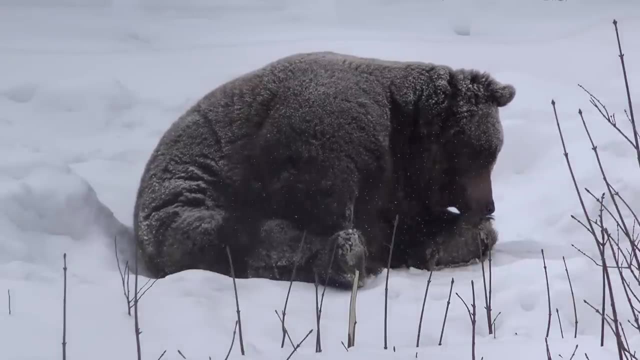 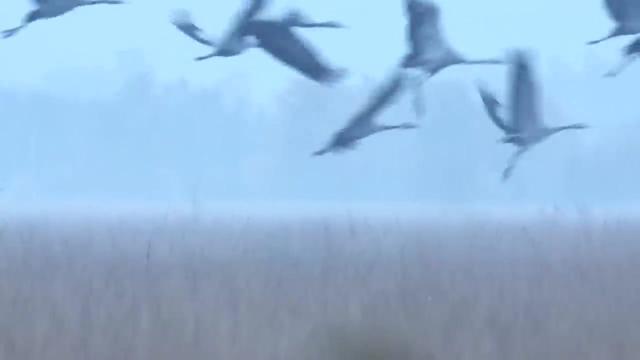 They keep all winter. if you can find a good hiding place, For some animals, winter is a time for hibernation. Hibernation: Some birds migrate, Others stay. Coniferous trees stay green all year round. Not many animals can eat their needles. 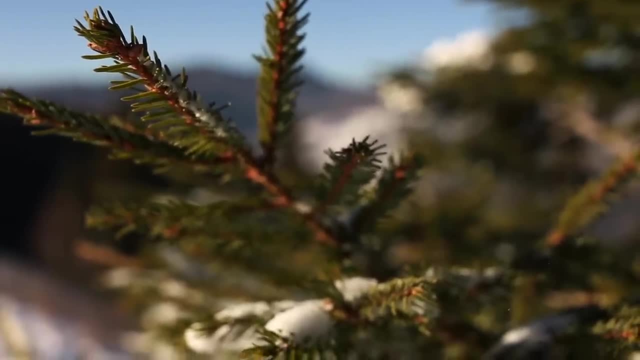 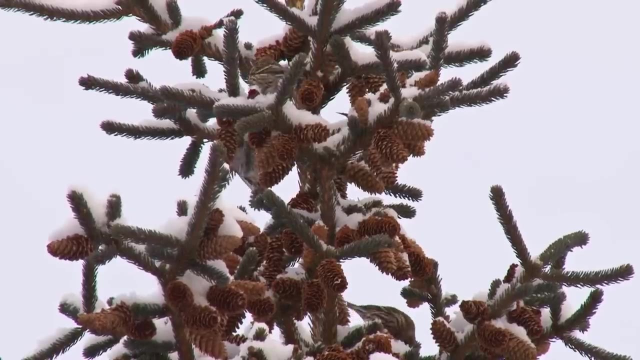 But their cones are packed with delicious seeds, As long as you can get to them With a beak or claws. The deciduous woods changes colour throughout the year, And the trees are growing. They are growing, They are growing, They are growing. 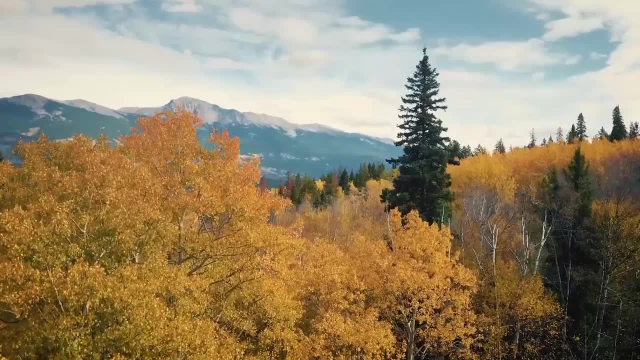 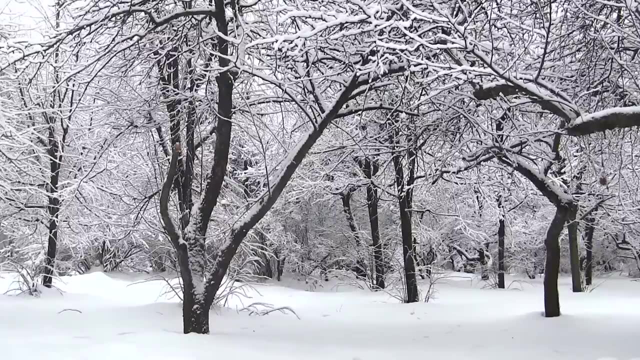 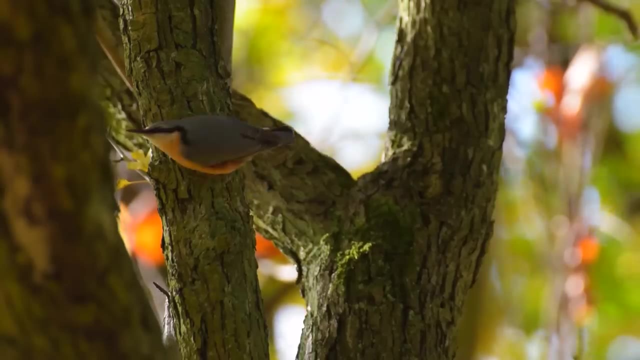 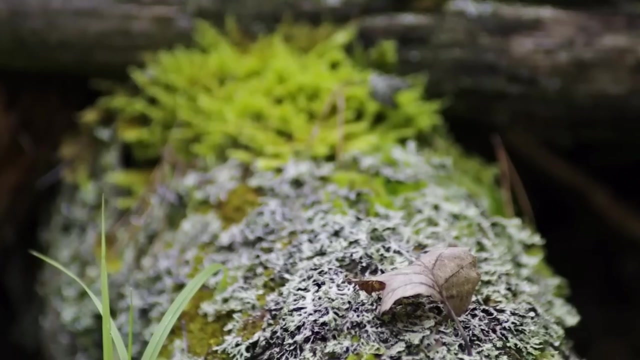 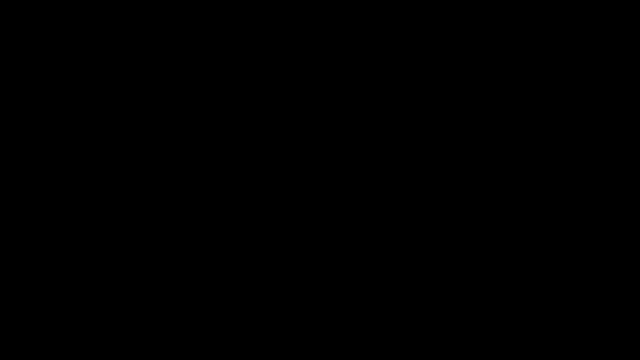 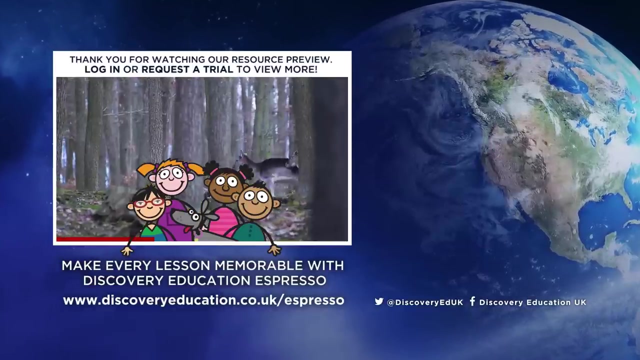 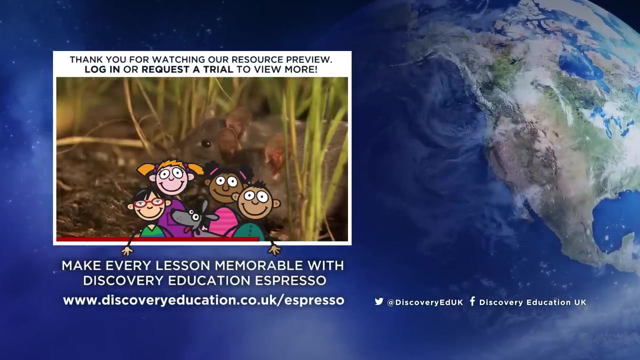 And spiders live by the trees. Thanks for watching into your Discovery Education and Espresso service to watch the full video and download supporting resources and activities. If you're not a subscriber, visit discoveryeducationcouk to request a trial.